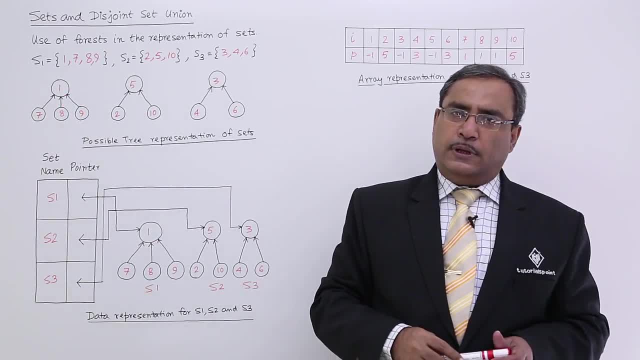 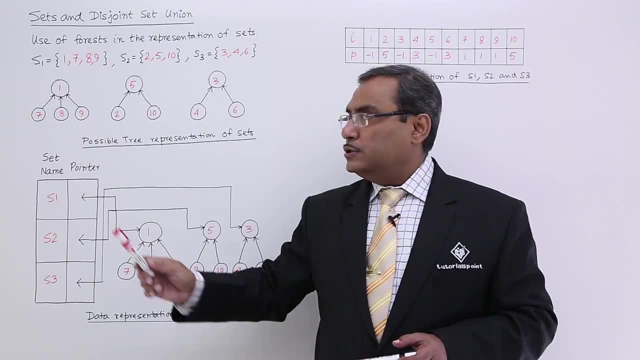 So in the root node, how many link fields we are supposed to keep, It is unknown, It is unpredictable. So that is why it is better to have that this children will be pointing towards the root, because all these children will have a single root and in this way the node formats can 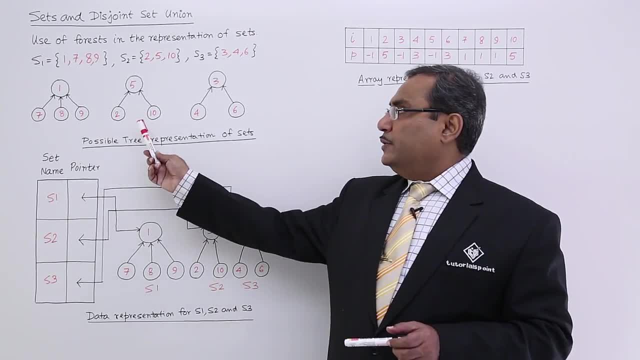 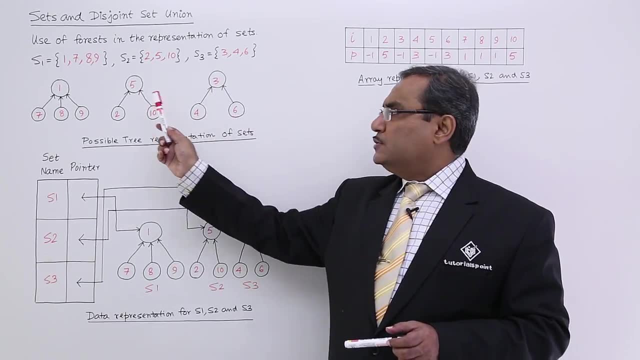 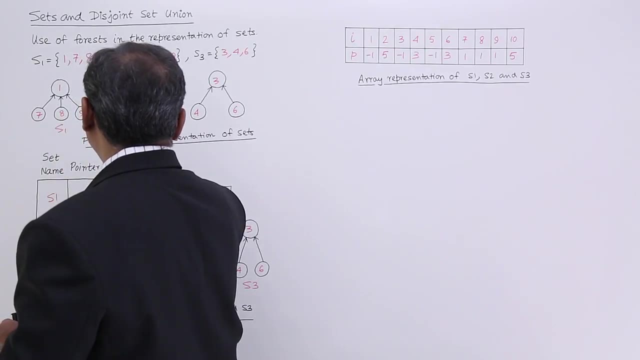 be easily reconstructed using the record structure. So in this case we are having this 2 and 10 pointing to this 5, and this 3 is being pointed by 4 and 6.. So set 1, set 2 and set 3, they have got represented. 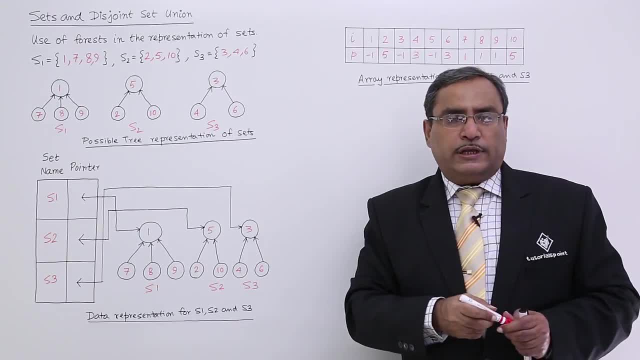 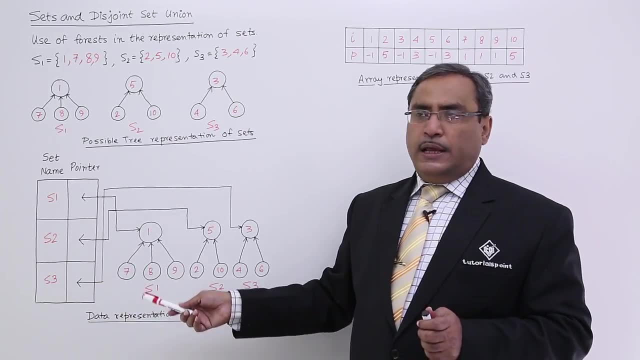 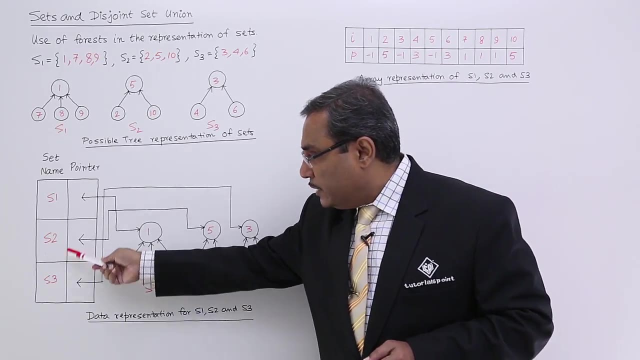 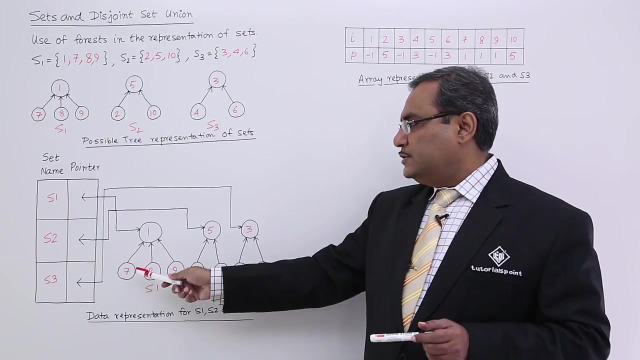 So here we are, using forest to represent these sets. So now there is another possible representation here. Here you see, this particular representation is good enough, but it is not holding the set names. So it is holding the set names. You see, this is the set S1 and it is pointing to this root node, and these are the children. 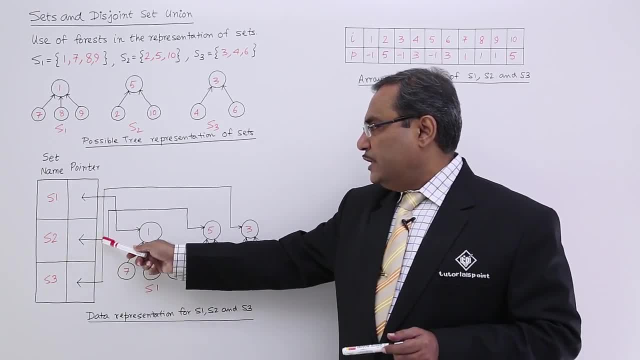 They are pointing to this root And this is my S2.. It is pointing to this particular set. So this is my S3.. This is my S4., This is my S5.. This is my S6., This is my S7.. 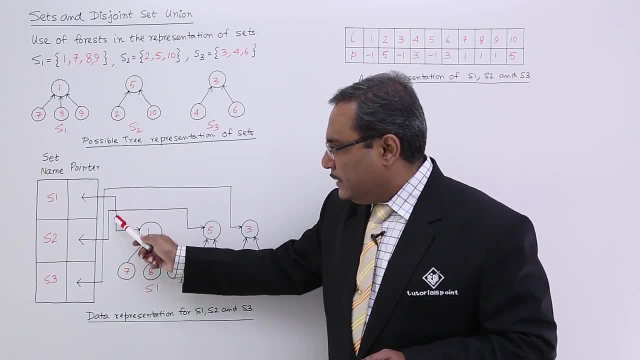 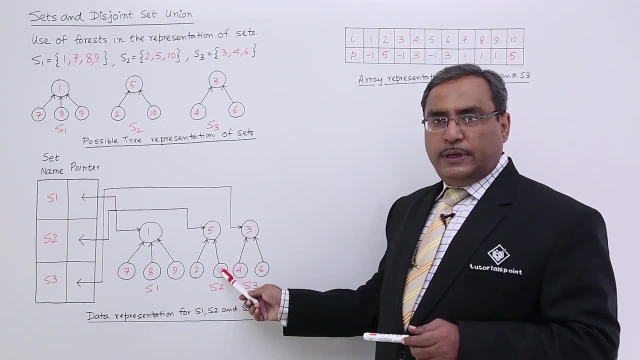 This is my S8.. This is my S9.. This is my S10.. And from here also you can move here, because the links are bidirectional according to the diagram given. So this 10 item is under which set? you can easily get that one because it is pointing. 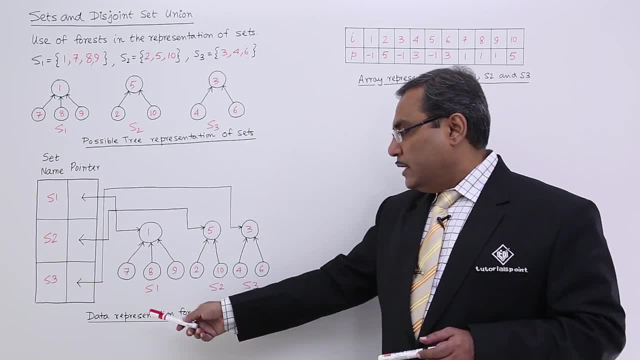 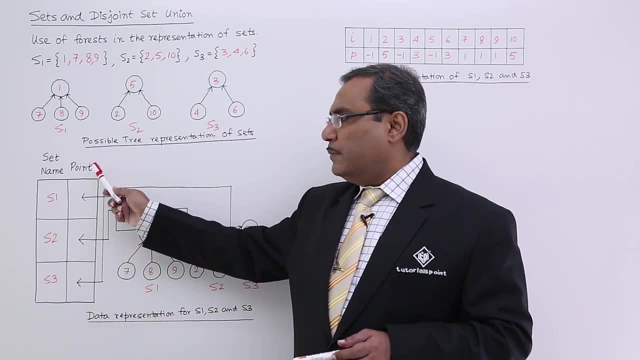 to S2.. So similarly, this S3 is there. So in this way the data representation for S1, S2 and S3 have got shown here. So we are having 2 columns here. One is containing the pointer and another one is containing the set name. but we can. 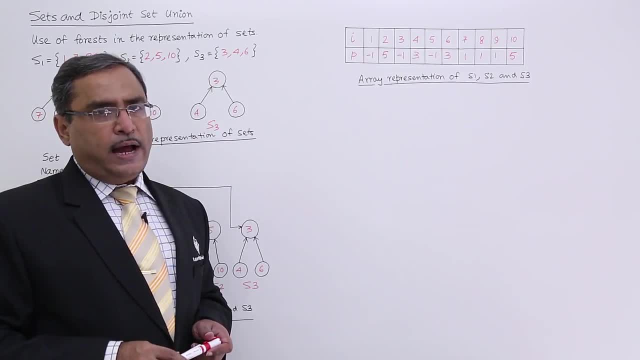 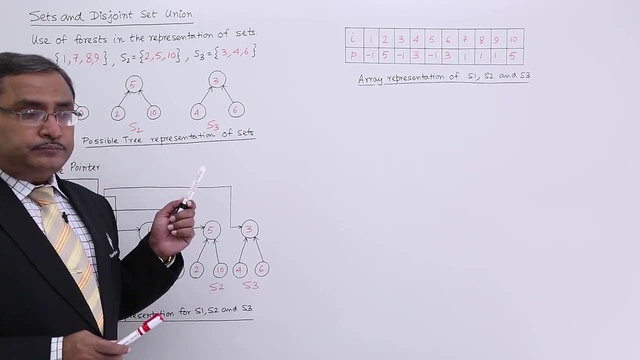 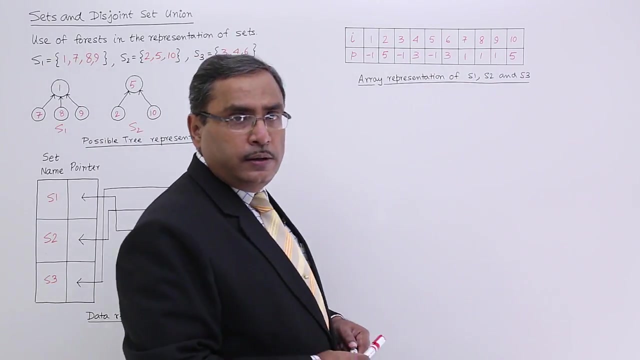 also have this array representation of s1, s2 and s3. so now, here you see how we represented this particular array. you see node number. node number 7, 8, 9 are having the parent 1. so 7, 8, 9, they are having the parent 1 and node number. this value, 1, is the root node, so this: 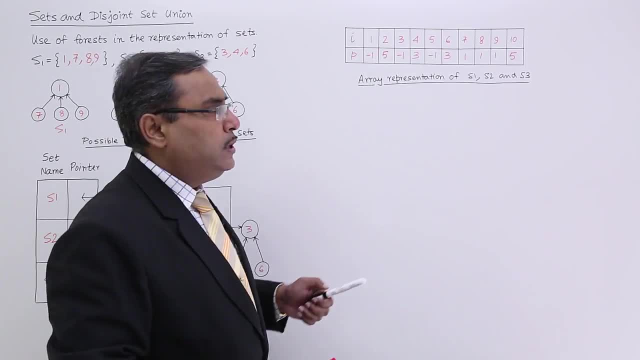 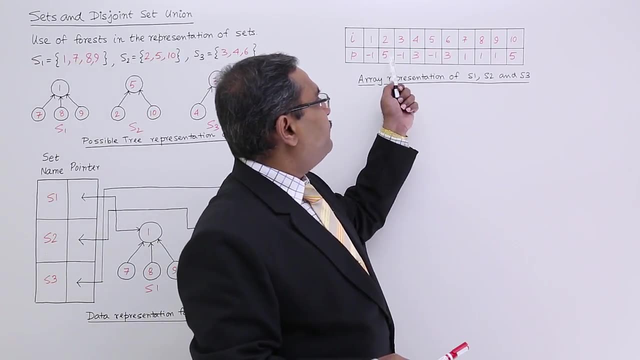 value 1 is pointing to no other node because it is a root. similarly we can go for 2 and 10 are having the root 5. so 2 and 10 are having the root 5. so 5 has been written and 5 is the root.